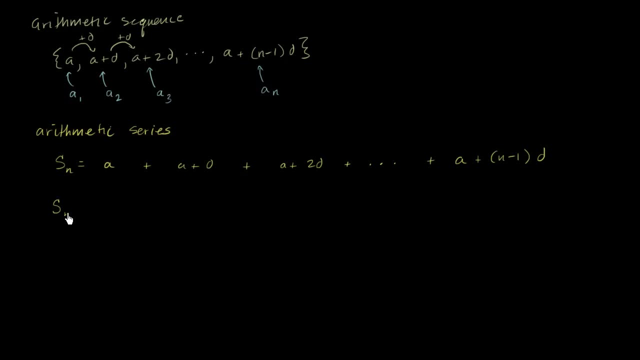 going to swap the order in which I write this sum, So the s sub n. I can write as this, but I'm going to write it in reverse order. I'm going to write the last term first. So the nth term is a plus n minus 1 times d. 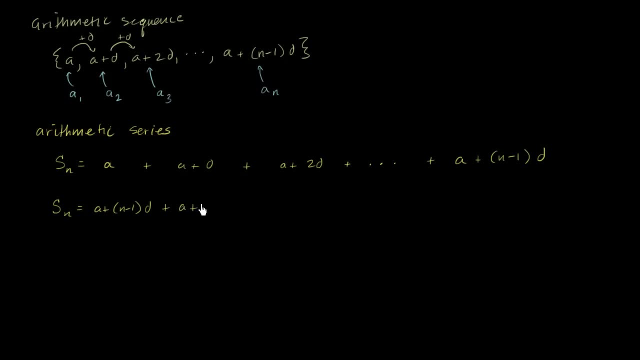 Then the second to last term is going to be a plus n minus 2 times d, The third to last is going to be a plus n minus 3 times d, And we're going to go all the way down to the first term, which is just a. 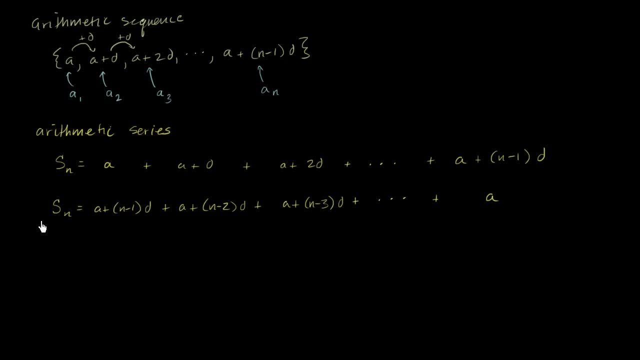 Now let's add these two equations. We are going to get on the left-hand side s sub n plus s sub n. You're going to get 2 times s sub n. It's going to be equal to well, what's? 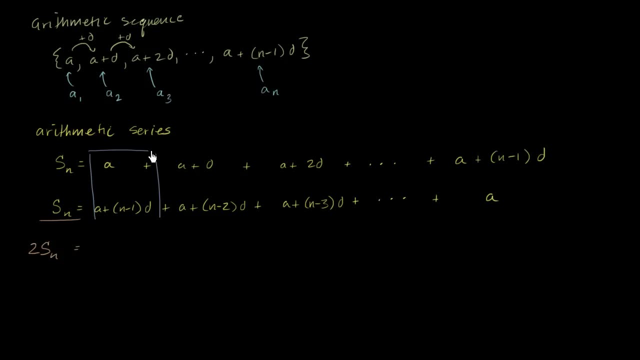 the sum of these two first terms right over here We're going to have a plus a plus n minus 1 times d, So it's going to be 2a plus 2a- OK- Plus n minus 1 times d. 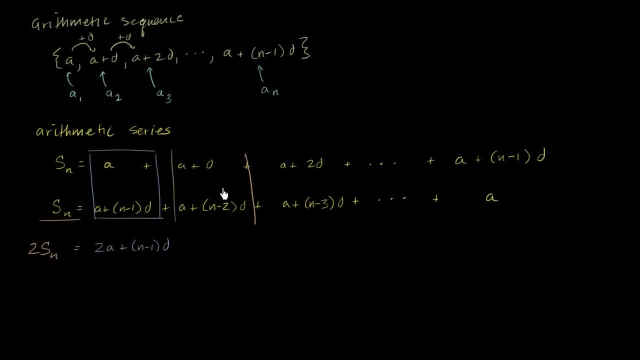 Now let's add both of these second terms. So if I were to add both of these second terms, what do I get? Well, I'm going to get 2a plus 2a, And what's? d plus n minus 2 times d. 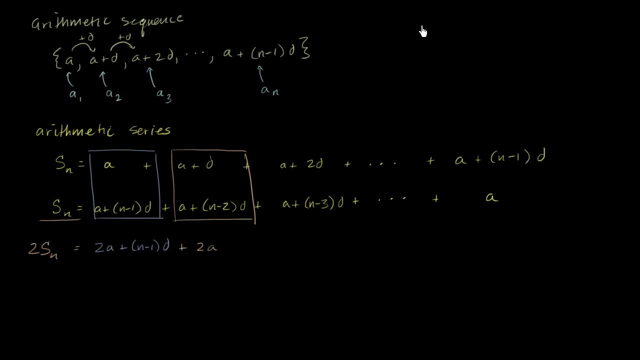 So you could view it several ways. You could view this. Let me write this over here: What is d plus n minus 2 times d? Well, this is just the same thing as 1d plus n minus 2 times d. 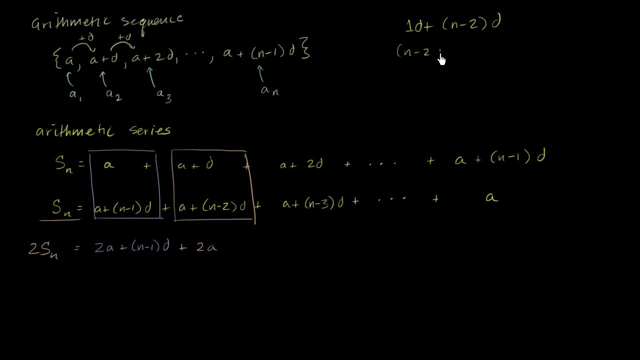 And so you could just write it like this: Let's just add the coefficients, So this is going to be n minus 2 plus 1 times d, which is equal to n minus 1 times d, So this second term also becomes 2a plus n minus 1 times d. 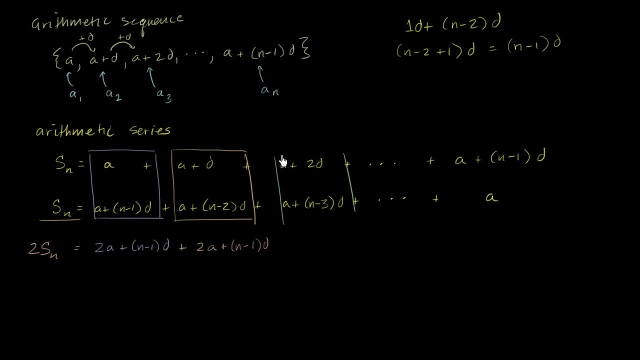 Now let's add the third term. I'll do it in green, or the third terms. I should say, And I think you're going to see a pattern here- It's 2a, So plus 2a. If I have 2 plus n, minus 3 of something, 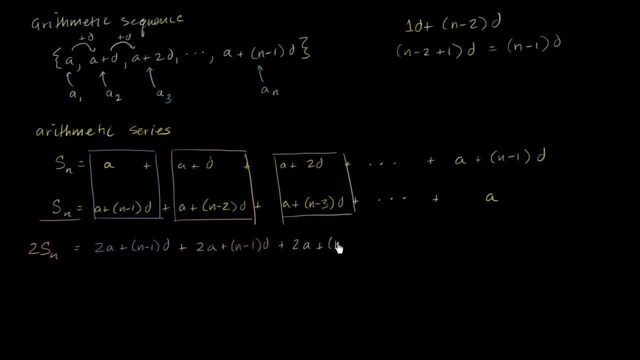 and then I add 2, I'm going to have n minus 1 of that something, So plus n minus 1 times d, And you're going to keep doing that all the way until your nth pair of terms, All the way until you add these two characters over here. 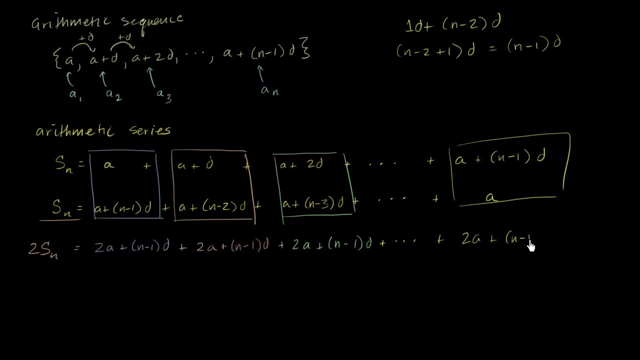 which is just 2a plus n minus 1 times d. So you have this 2a plus n minus 1d, which is equal to n minus 1d. Let's add that being added over and over and over again. 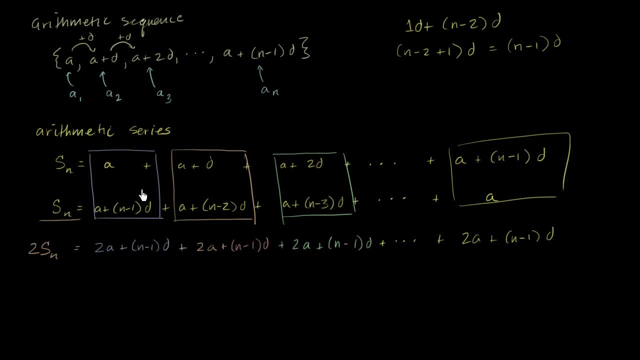 And how many times are you doing that? Well, you had n pairs of terms when you were adding these two equations, Or in each of them you had n terms. This is the first term, this is the second term, this is the third term, all the way to the nth term. 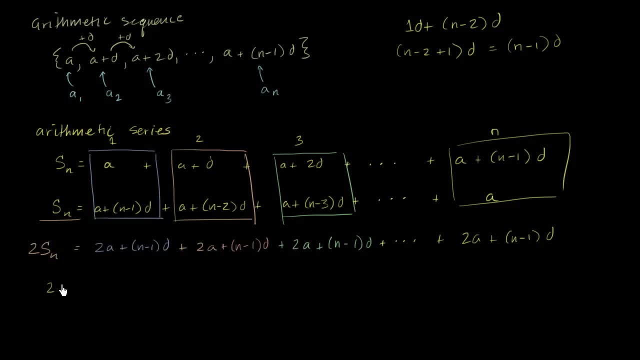 So I can rewrite this sum or the 2 times the sum, 2 times s sub n is going to be n times this quantity. It's going to be n times 2a plus n, minus 1 times d, And then if we want to solve for s sub n, 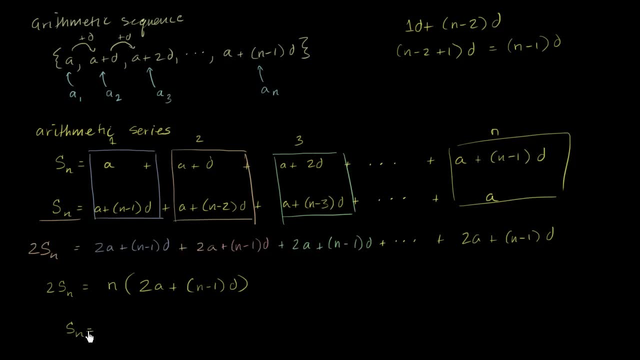 you just divide both sides by 2. And you get s sub. n is equal to- and we get ourselves a little bit of a drum roll here- n times 2a plus n minus 1, times d, all of that over 2.. 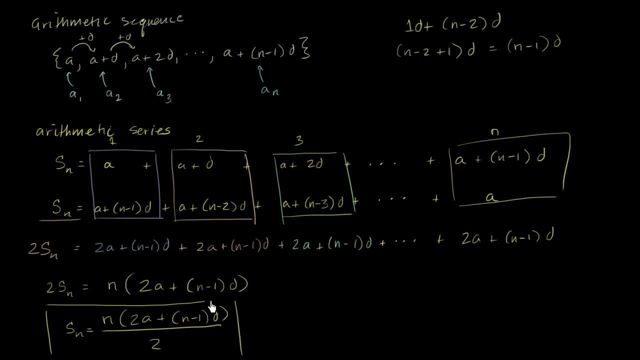 Now we've come up with a general formula, just a function of what our first term is, what our common difference is and how many terms we're adding up. And so this is the generalized sum of an arithmetic sequence, which we call an arithmetic series. 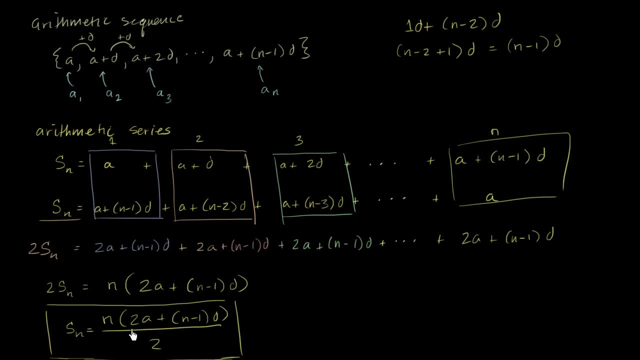 But now let's ask ourselves this question. This is kind of hard to remember. You know, n times 2a plus n minus 1 times d over 2.. But in the last video, when I did a more concrete example, I said: well, it looks like an arithmetic sequence. 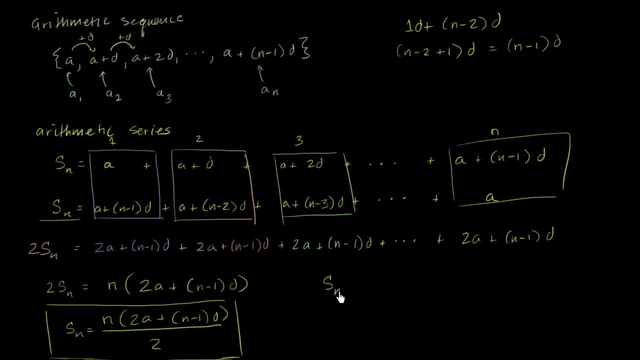 It looks like the sum of an arithmetic sequence could be written as perhaps could be written as the average of the first term: a1 plus an, the average of the first term and the last term. So that's the average of the first term and the last term.